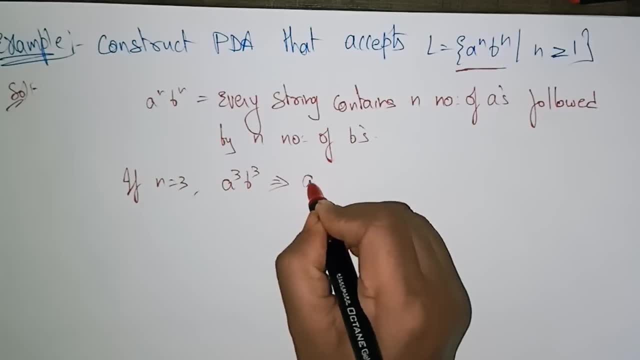 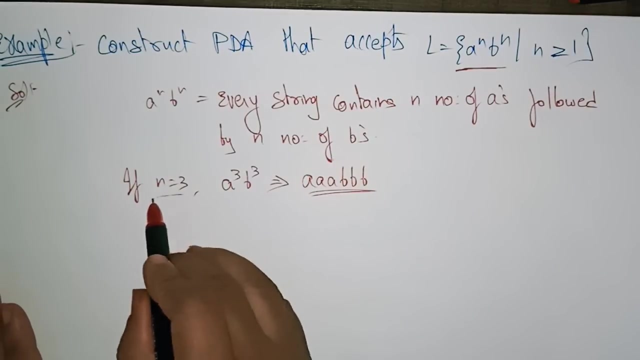 a cube, b cube. that is nothing but a, a, a, b, b, b. So means the string should be like this: a a, a, b, b, b. Okay, so now let's see. now let's construct a PDA that accepts this string, or not? Okay, let's take: n is equal to 3.. So with whatever, 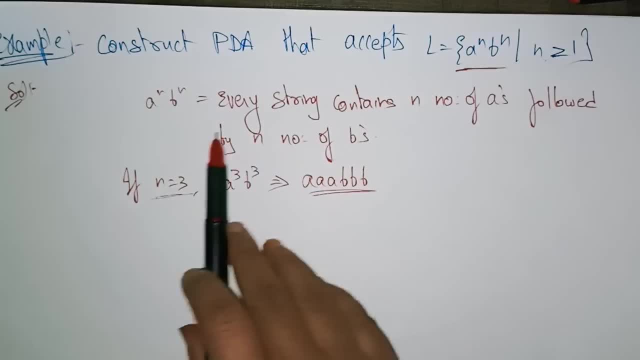 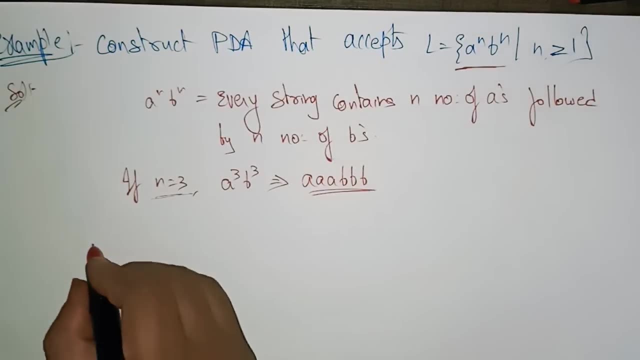 the value you want, you can take, but it should be greater than or equal to 1.. Don't take 0.. Okay, the string has to. the n has to be started from 1 onwards. Okay, so let's initially, the stack is: 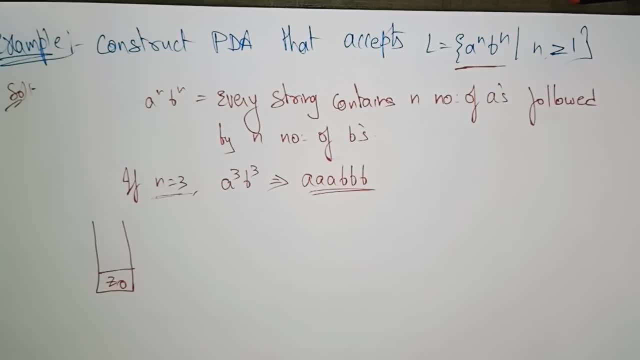 empty Means z naught represents the empty stack. Okay, the stack is empty. First thing is, if we uncount, first input is what is the first input? So I have to please, So finally I have to again come back with the z only of z naught. Okay, so after reading the entire input string, the final, 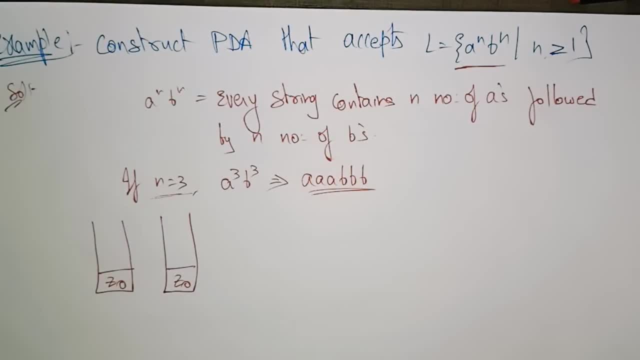 thing is I have to get the empty stack. There is a empty stack acceptability. So I said the PDA can be accepted by using two ways. One is a final state acceptability and another is an empty stack acceptability. So in this video I'm taking one of the way. that is empty stack. 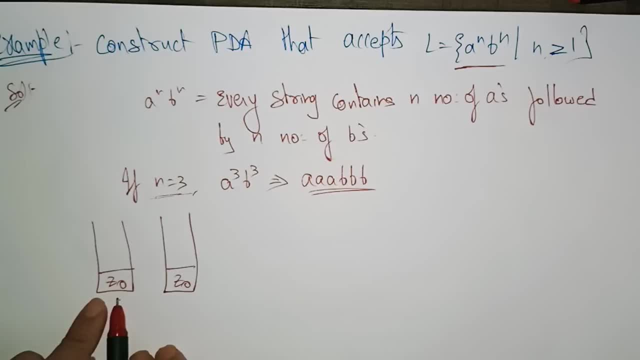 acceptability. So the first, the first string here we have taken is a z naught. the stack is empty. So first you need to push a, push a on to the top of this stack. So whenever, if you uncounted, input a the top. 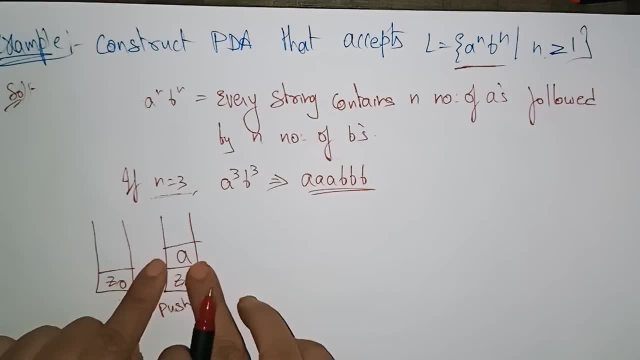 is null. okay, the top is null, then we have to push a onto the stack. okay, push a onto the stack so this may be iterated. means how, if suppose any number of a's that has to be iterated here- in this example i have taken n- is equal to 3, means total 3 a's has to be pushed onto the top of the. 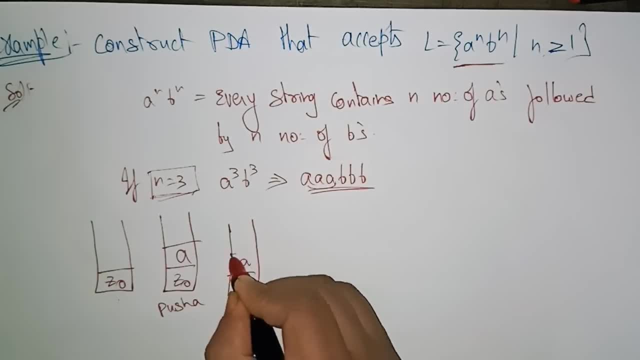 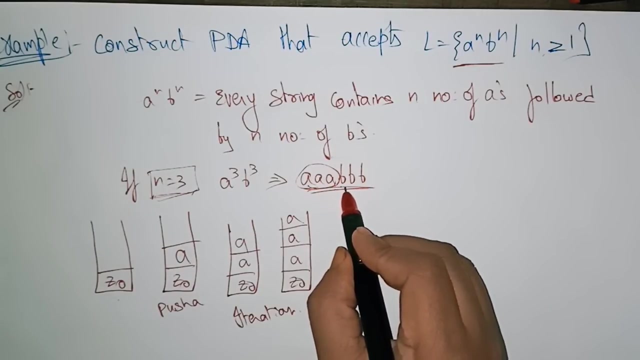 stack. let's push that. okay. z naught a- a, so i push the a. and again, z naught a, a, a, so total 3 a's i pushed onto the stack means i've done the iteration here, iteration- okay. so now, if we, the next element that i have to read is a- b. so whenever i encounter the input b. 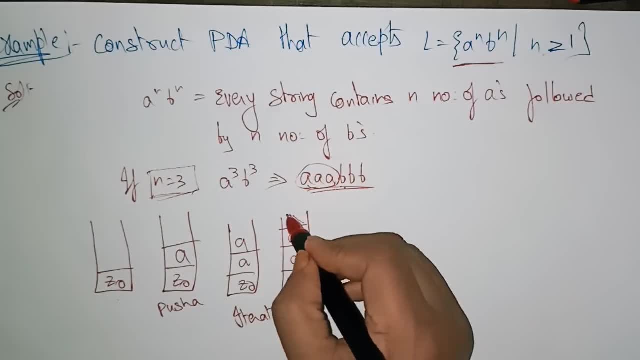 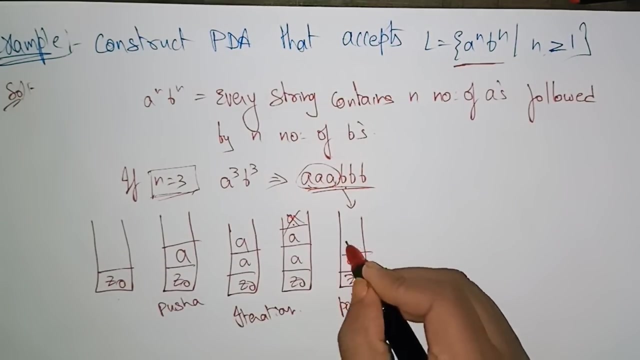 the top, a has to be popped. this has to be popped. so whenever i encountered b, okay. whenever i encountered b, b, pop a on top of this stack. now it contains only again: whenever i encountered b, i need to pop the topmost element. pop a. okay, whenever i encountered b. 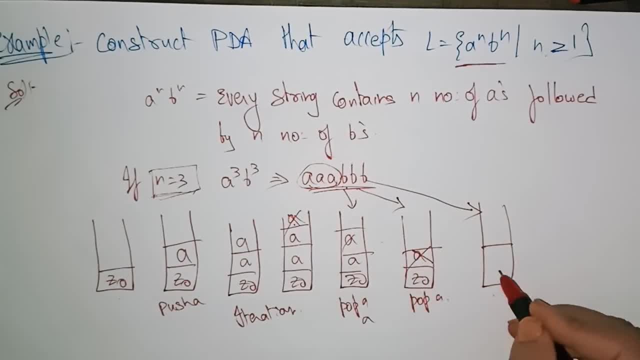 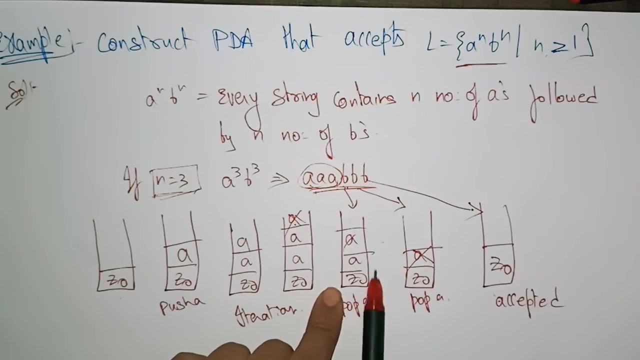 okay, pop the topmost element now. it contains only z naught, only contains z naught. so that means it is accepted. uh, because i read the complete string. okay, so the first. whatever the element, that is, same elements are there. you need to push the elements on the top of this tag. okay, whenever you encountered 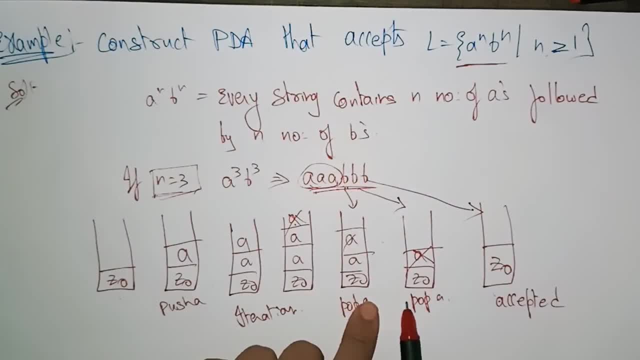 a different input element, then you started the popping. okay, the three elements has to be popped. the final thing you have whenever you reach the z naught: whenever you reach the z naught, if the string is completed, then the string is accepted. suppose, if the string is not completed, 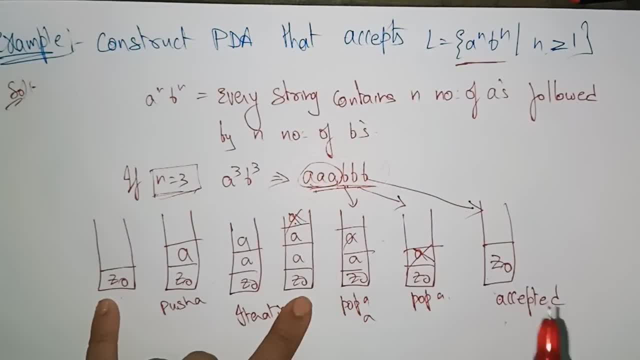 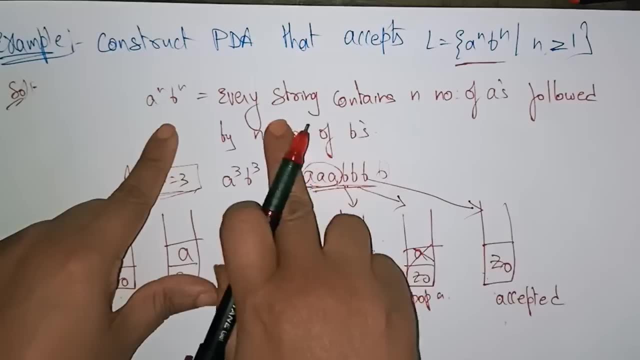 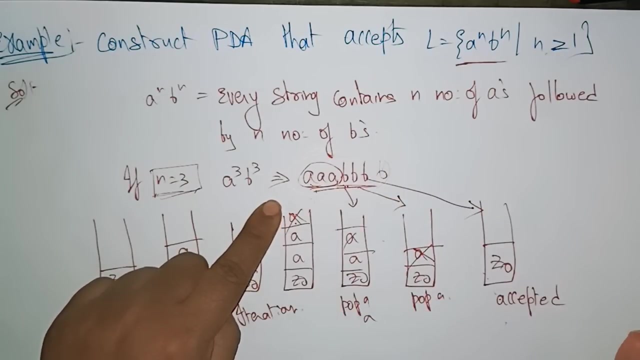 if the string is not completed then you can say it is not accepted. suppose if take another b you have taken, but we have to get the equal number of a's and equal number of b. suppose a cube and b4 you have taken. but it is not our concept, because it should be equal number of a's and equal number. 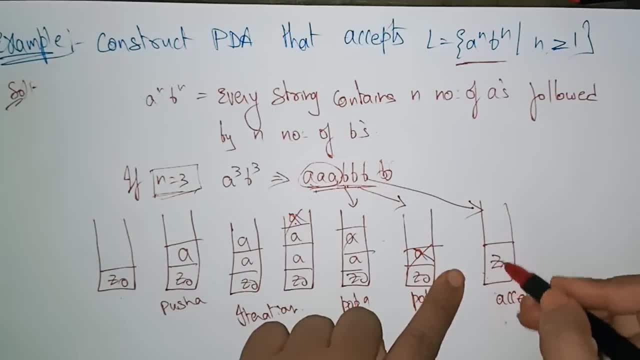 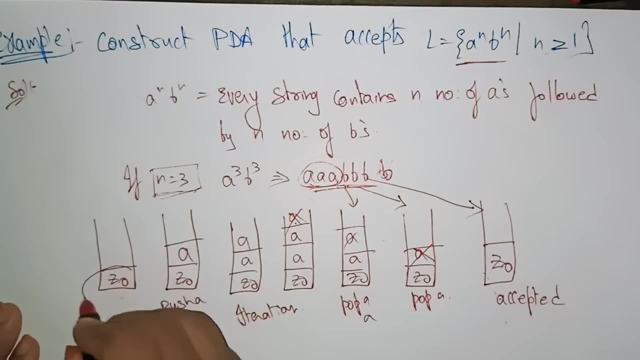 of b. if i take a, one more b: okay, but there is no element that has to be popped onto the stack, so the string is not accepted. but here, in this case, the string is accepted because the stack becomes empty. so this is a technology. okay, let's see the transition diagram for this. 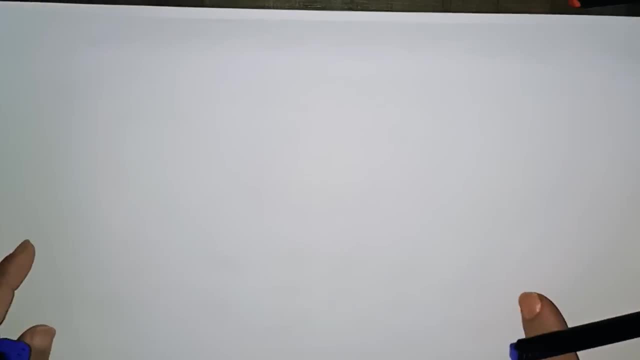 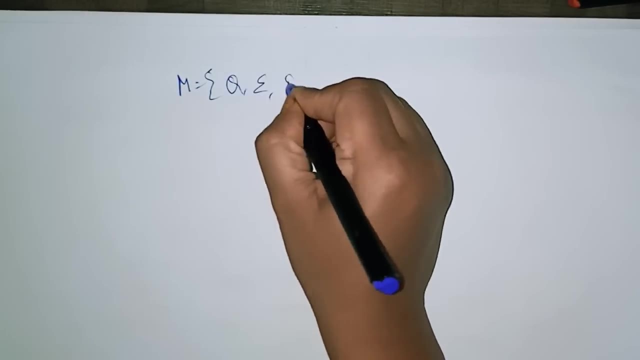 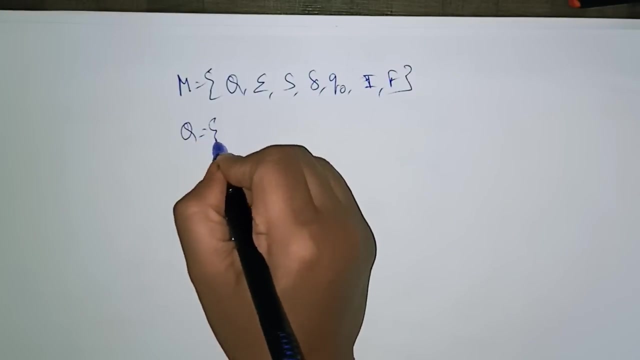 for the given, whatever the language that is there. so you know that, ml. let's take the language q, sigma s, delta, q, naught i, comma f. so the q is nothing but the set of states here: q naught, q1 and the q2, 2, 3- total three states are there because we are taking the string. 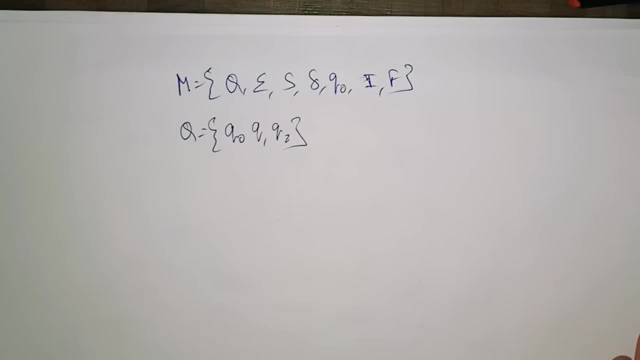 okay, the string a- b. whenever the two strings are there, the state has to be three. okay, from starting onwards i'm taking that, whatever the input values that you are taken. so the input values is n, the number of states becomes the n plus 1. so whenever the input values 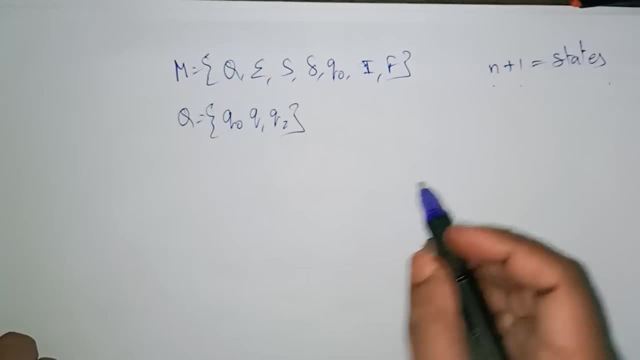 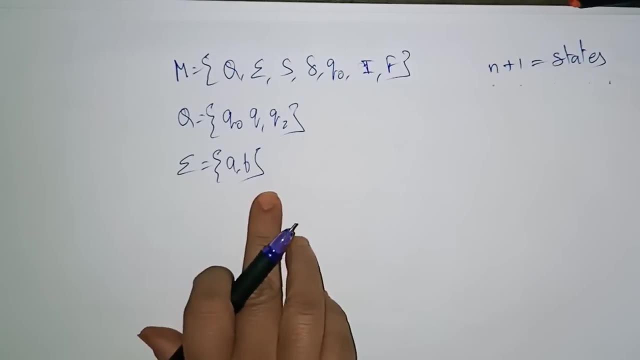 is n, the number of states becomes n plus 1. so here the input values, that is, a and b, are there, that is, the sigma is nothing but sigma is a, b. so whenever the sigma is ab means the number of states becomes 3, q, naught, q1, q2. and what is the final f should be: 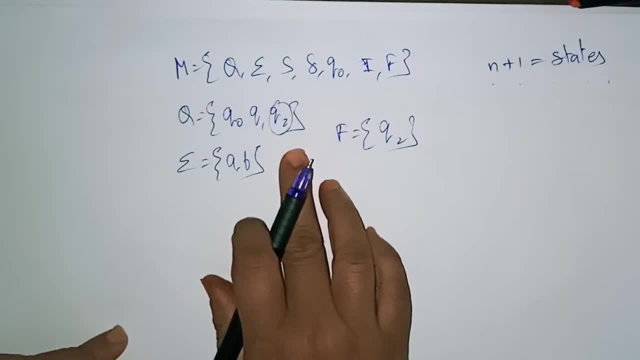 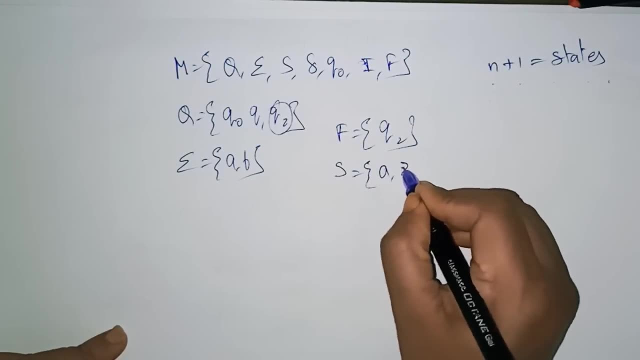 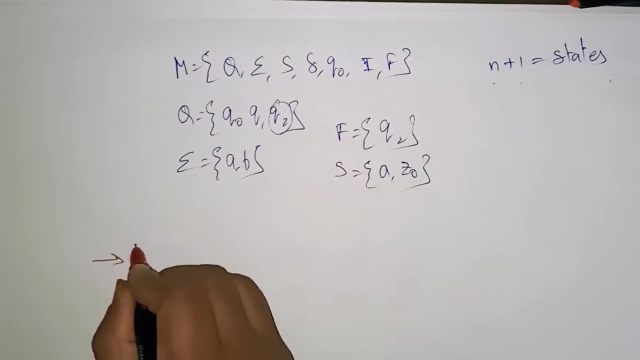 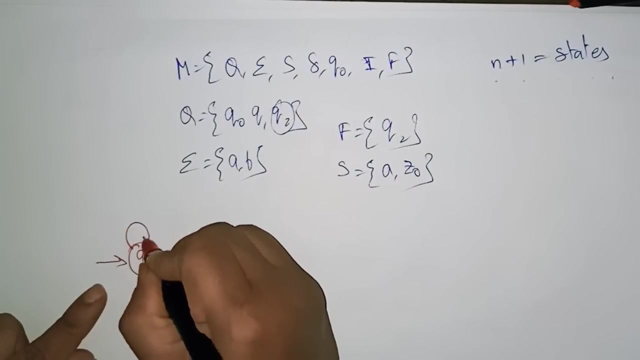 the final state should be q2- okay and s. the stack contains. what is the stack contains? the first, the stack contains the start symbol and the empty. now start the transition diagram, how it will be represented. so first it is q- naught okay in. q- naught okay, the first. whatever the input, what? 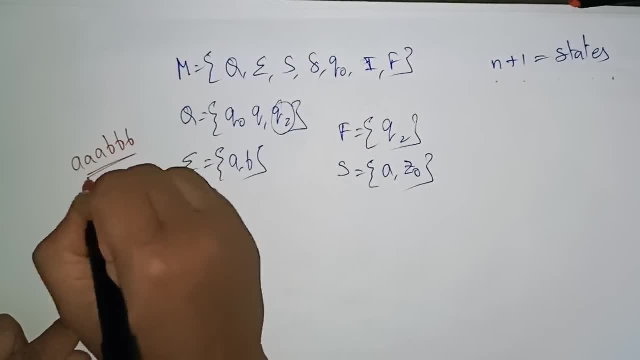 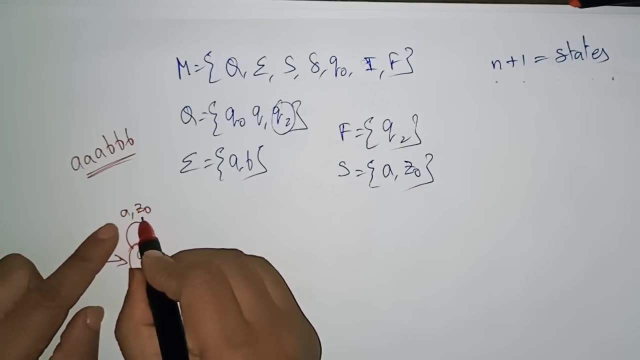 is the string a, a, a, b, b, b. so this is our input string. so whenever the input a is encountered and the start top of the stack is z naught, top of the stack is z naught, then push a onto the top of this stack. so again, 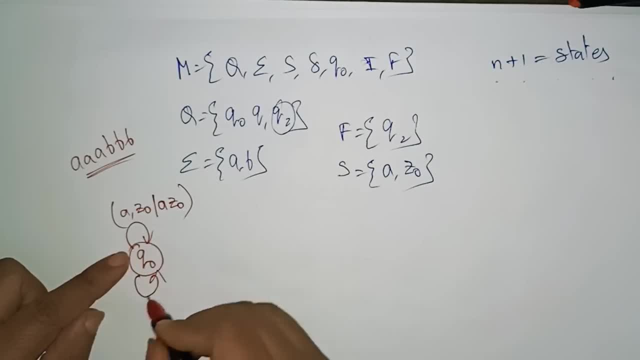 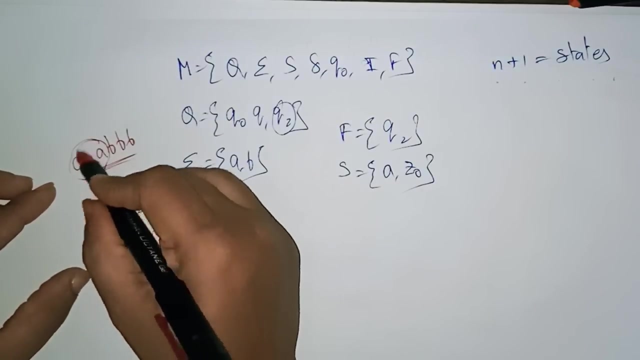 q naught. so in the same q naught state: only: okay. so whenever the top of the stack is, whenever the input again it is a. now the top of the stack is a. okay, you place a on the top of the stack. so this is until all the a's that are read on the top of the stack. so now i encountered 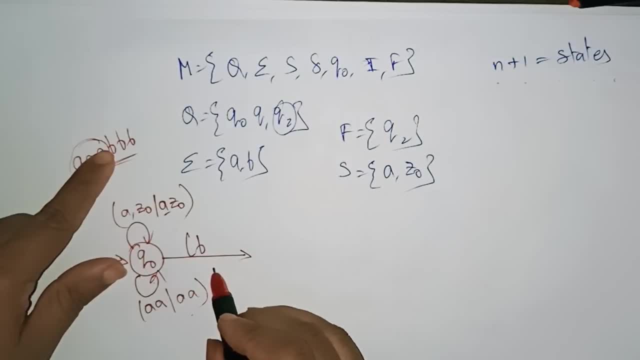 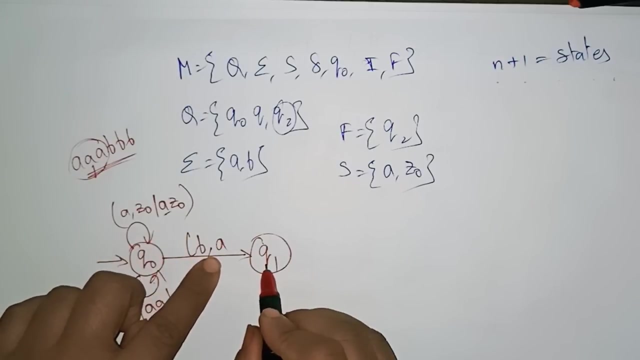 element b. so i encountered an element b. so whenever the element uh, whenever i encountered a new uh input b, b, input element b, i have to change the state, that is, i change the state to q1. so whenever i encountered element b, the a has to be popped. the a is the element that i need to be popped. popped means: 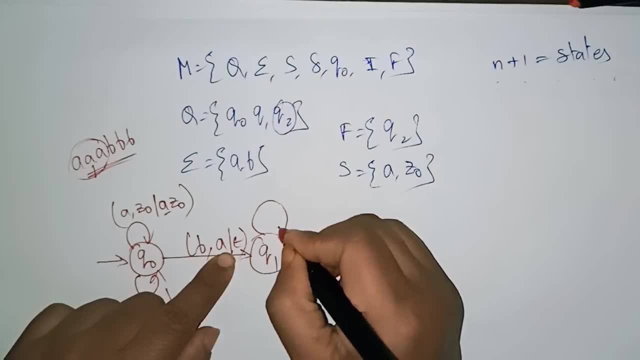 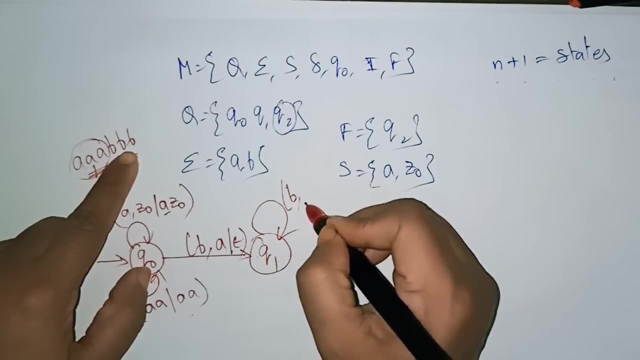 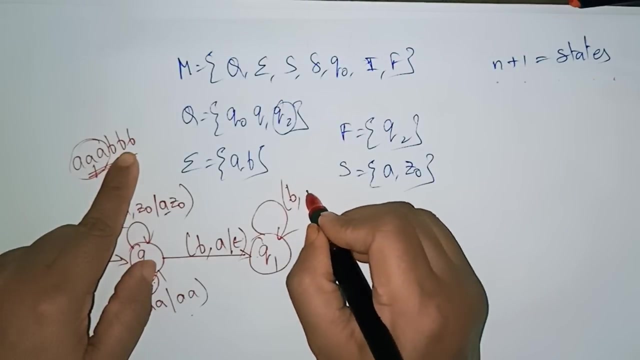 sigma epsilon. you have to write, so this has to be repeated. this has to be repeated. this is for one b and this has to be repeated based on how many. how many b's are there? still two b's are there, so the b has to be input and a has to be popped on the stack. so whenever the 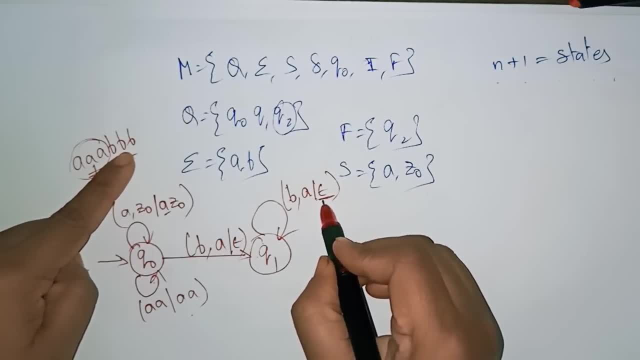 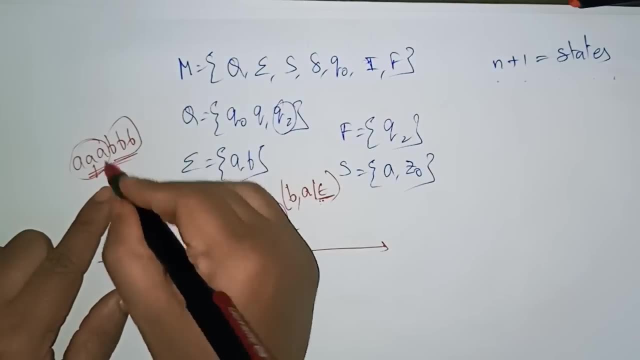 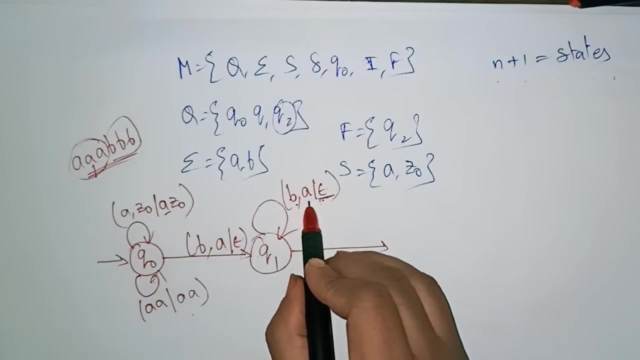 popping should be there, you need to write the epsilon here. whenever popping should be there, you need to write the epsilon. okay, so now i i read all the input strings b, all the inputs elements b. okay, and i popped all the a. a are completely popped now that state. 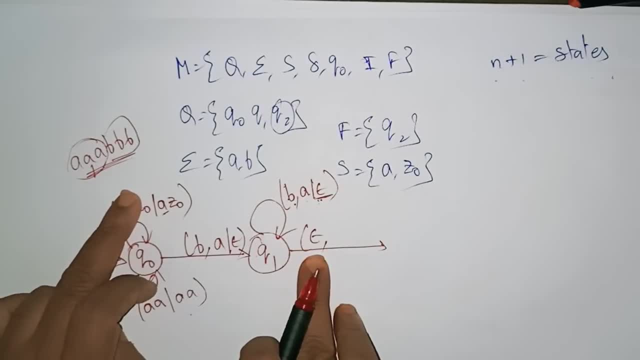 uh, the stack contains means that there is no input string that i have to read, so that's why i have written: here is epsilon, okay, and the top of the stack contains a z naught, okay. this is the stack contains z naught. top of the stack is z naught. now the stack contains z naught because everything is. 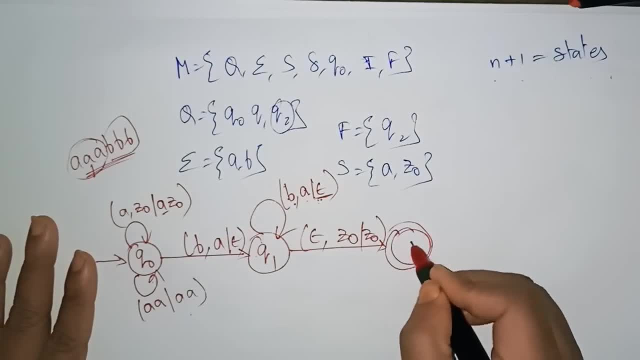 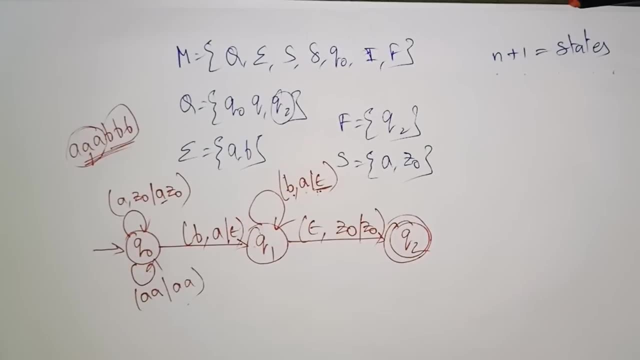 empty. okay, nothing is there. so then it reaches to the final state. so now the pda accepted by the final state. so this is how you have to represent the pda transition diagram based on language. it's a symbol. if you know the id concept, then you can easily. 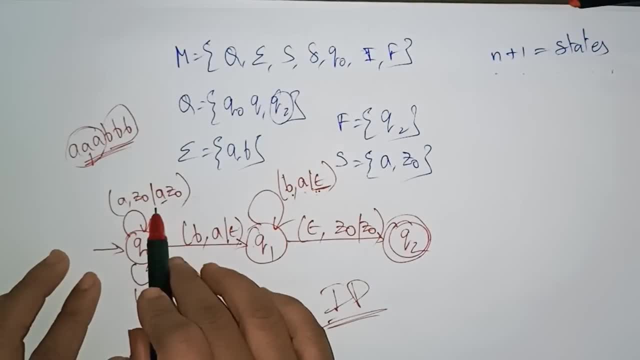 draw this diagram and you can understand these elements, okay. so this is very simple. whatever the elements that you are taken, so that can be. uh, so here, this is an input. this is an input, okay. stack contains number of a's- whatever the number of is. that will be there, okay, and here. 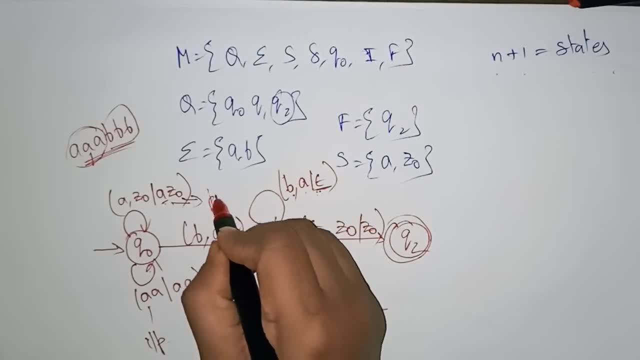 whatever the a that is there, that you are, you need to be push onto the stack. these elements that you need to push onto the stack. this is all epsilon. so you need to push onto the stack. this is the line. there is no, we are nothing to push on the stack, we are just popping. we are nothing to push. 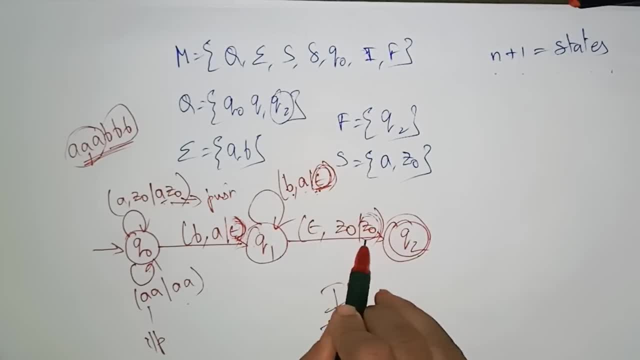 on the stack. we are popping. okay, we are nothing. to push onto the stack, this nothing. it's an empty string that represents. so this is about this pda. so we'll see one more example in the next video. thank you.